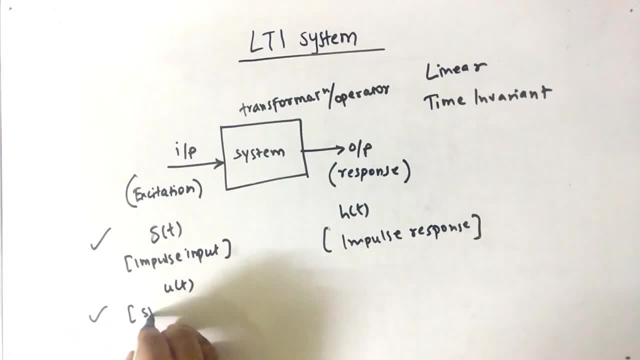 function we have is u of t. Now this is known as the step input. If we give the step input, we get the step response, So this is known as the step response. So these are the important terms, like impulse input, impulse response, Step input, step response, And this transformation is done by the. 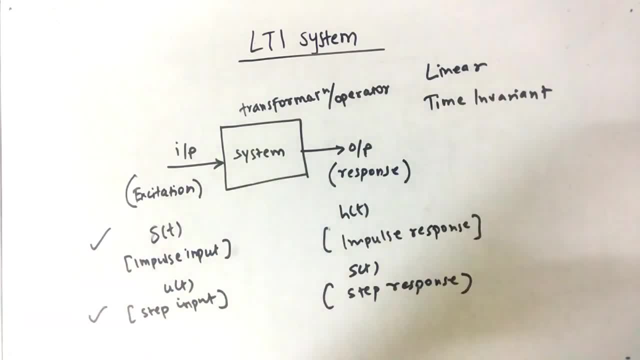 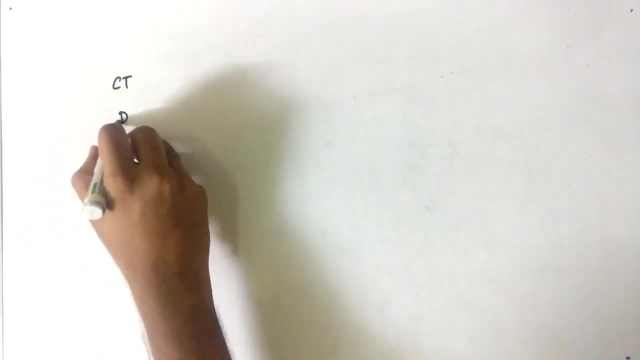 LTI system. So this is the important concept. Now let's look at the properties of LTI. First, we will talk about the signals. We have two types of signals: continuous time and discrete time. If we talk about continuous time, we will talk about the t notation. If we talk about discrete time, we will 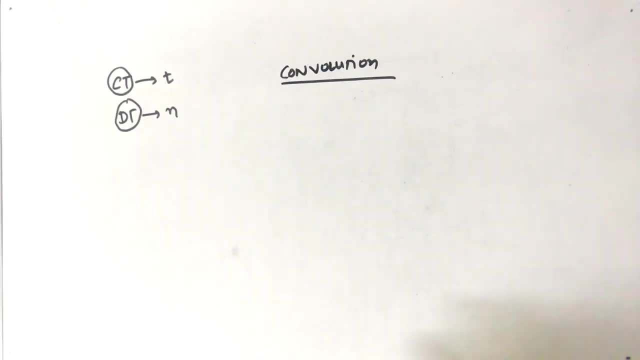 talk about the t notation. So now let's talk about convolution. When we talk about convolution, we are trying to find the output. So we are basically finding output. If we talk about the continuous time, we are finding y of t. If we are talking about discrete time, we are finding y of n. So let's talk. 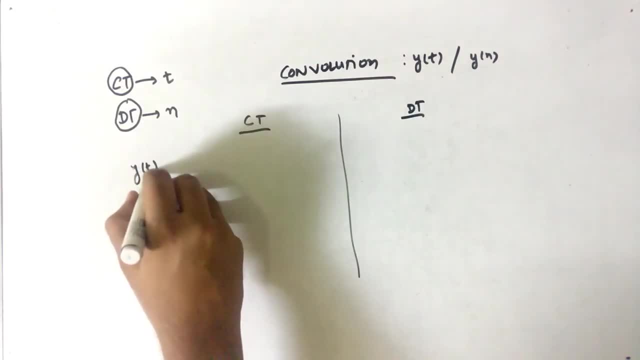 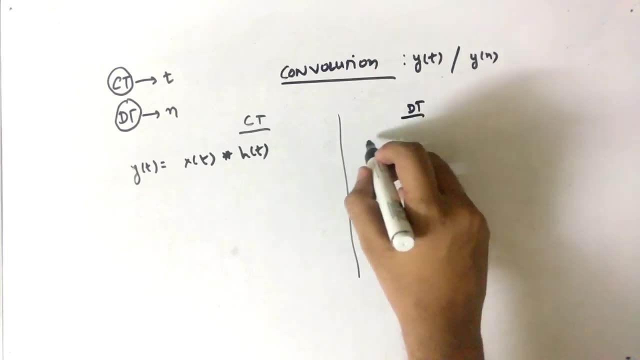 about the continuous time. first, If you have to find y of t, you have to convert two functions. That is, x of t is converted with the h of t, Simple And in discrete time the notation would be n. So y of n is equal to x of n. 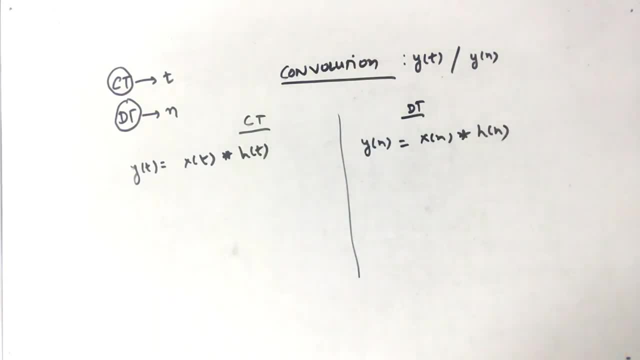 Converted with h of n. Now if we talk about convolution formula, the formula is: y of t is equal to integral minus infinity to infinity x of tau, h of t minus tau d tau. Or it can be integral minus infinity to infinity x of t minus tau h of tau d tau At the end overall of this bracket. 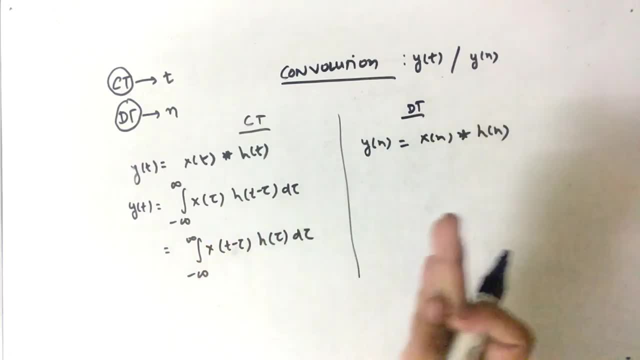 should be t, Like tau plus t minus tau. Answer is t. So both are the correct formula. It's upon you how you want to use. If we talk about discrete time, we will use the summation, So this is important. When we talk about continuous time, we are using. 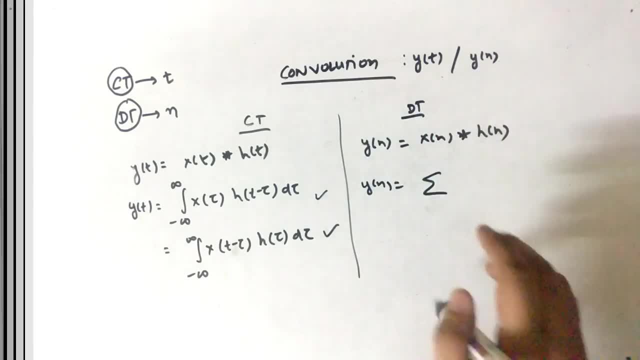 the integral, But when we talk about the discrete time we are using the summation. So the formula for discrete time is: y of n is equal to summation, m is equal to minus infinity to infinity, x of m into h of n minus m. So this was about the convolution. 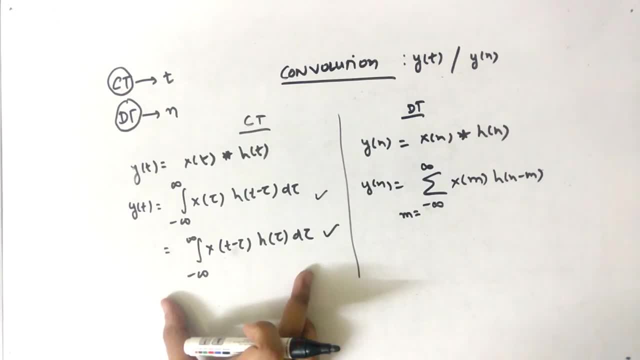 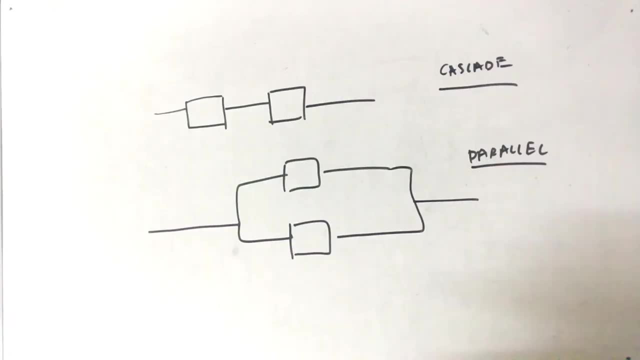 Now this is important for both gate examination and academic paper. One question is sure on this formula: Convolution formula. Now the next point is about how they can manipulate h of t, That is, the impulse response. h of t means the impulse response, Alright, So 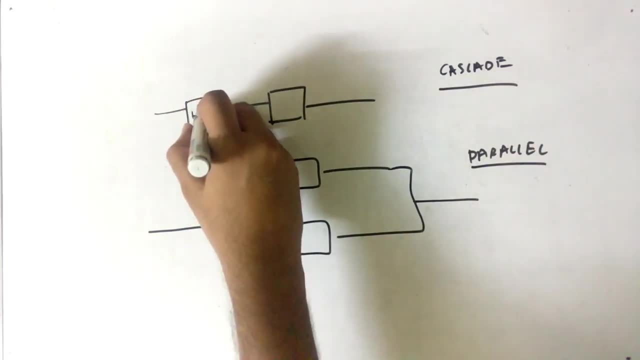 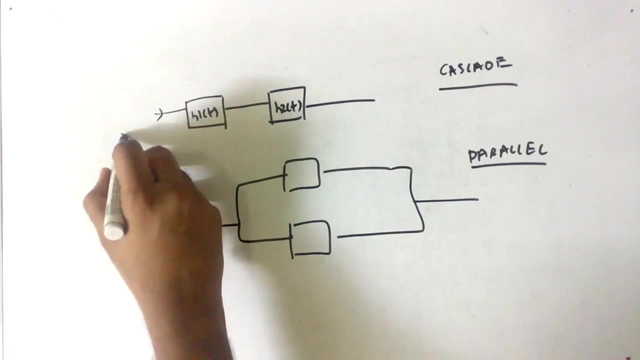 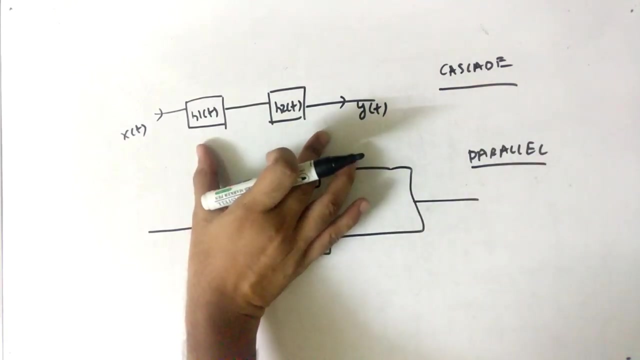 there are two types they can manipulate. First is suppose I have h1 of t and here I have h2 of t. Now they are connected in series And here you are giving input, that is x of t. So what is the impulse response here? So the impulse response would be: h of t is equal. 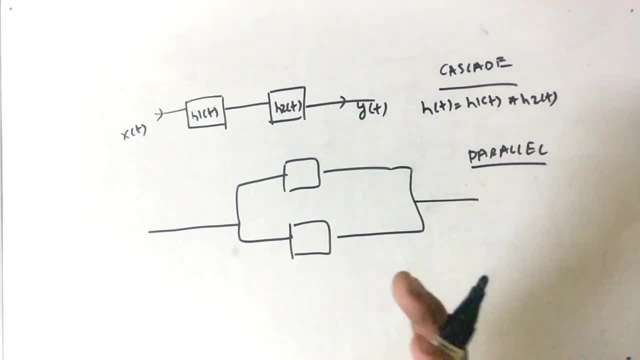 to h1 of t convolved with h2 of t. So whenever they are in series, like two impulse response are in series, then you can say that complete overall impulse response is equal to h1 of t convolved with h2 of t. Now let's talk about parallel. Now again we have the input x of 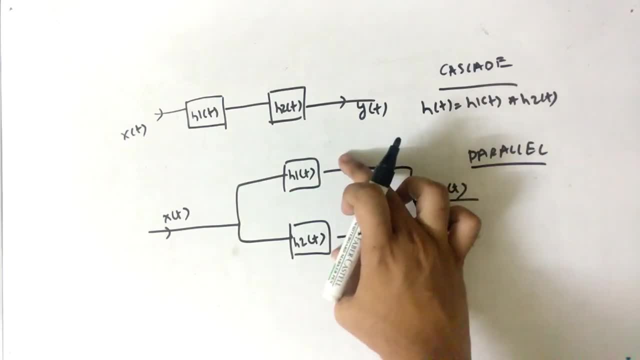 t, We get the output y of t. Now the two impulse response are h1 of t and h2 of t. So h1 of t and h2 of t are connected in parallel. If that is the case, then the complete or overall. 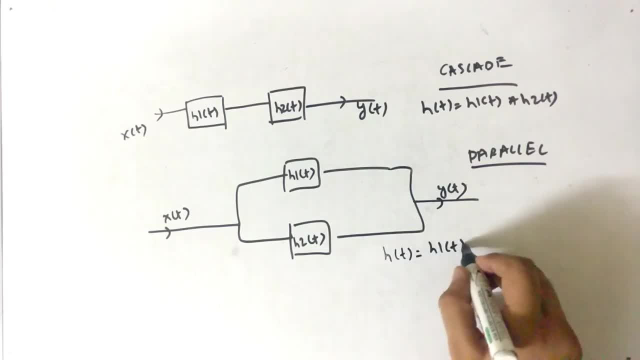 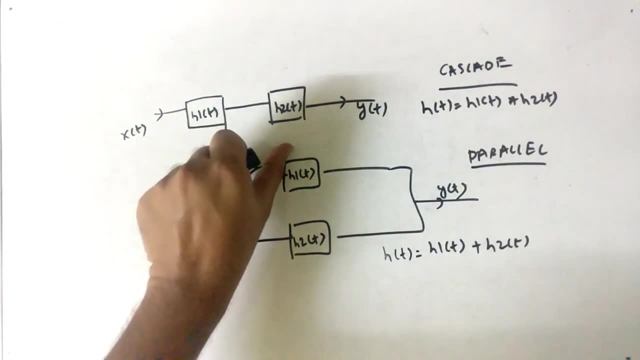 impulse response is h of t and that is equal to h1 of t plus h2 of t. So this is important. the concept of cascade: This means that two impulse response are in series. You have to convolve that. The concept of parallel: You have to add those. So this is important. Now, 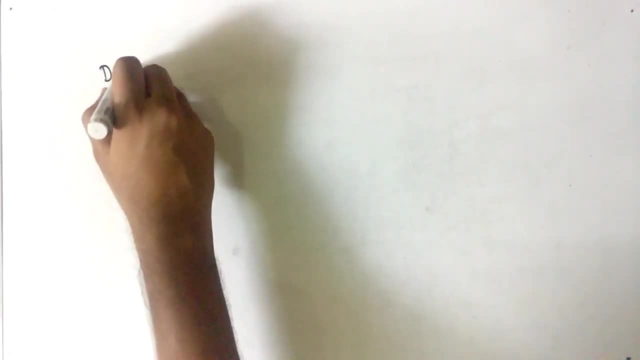 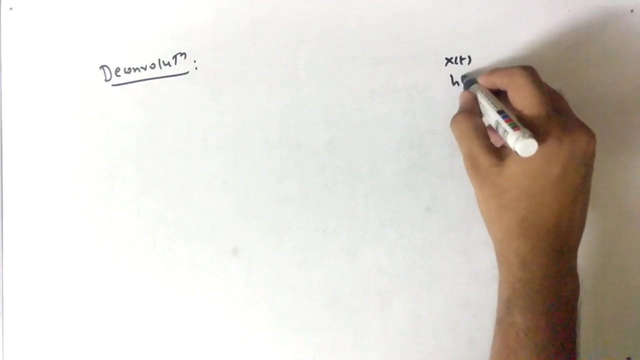 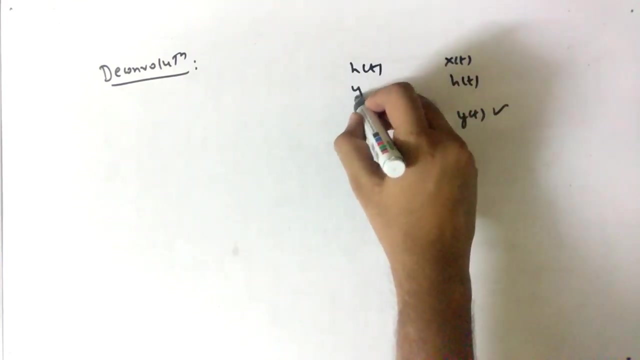 let me introduce you with some terms. The first term is deconvolution. Now, this is important Deconvolution. When we talk about convolution, we had x of t, we had h of t and we found y of t Correct. Now, in deconvolution, we will have h of t, we will have y of t and we will 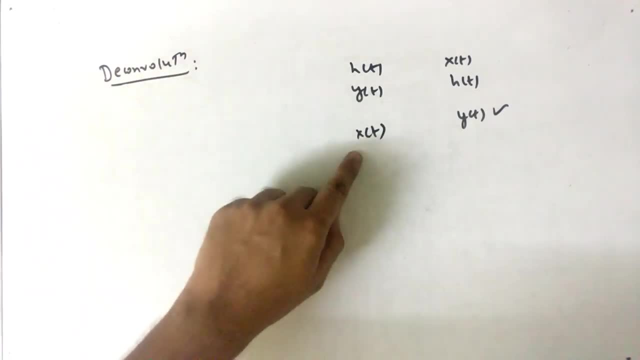 find x of t. So deconvolution means finding x of t from y of t. Now let's talk about identity system. Now, what is that If you have a system in cascade with the inverse system? So what I meant is you have a system. 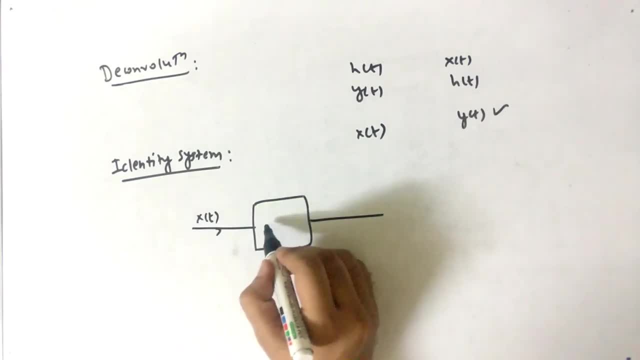 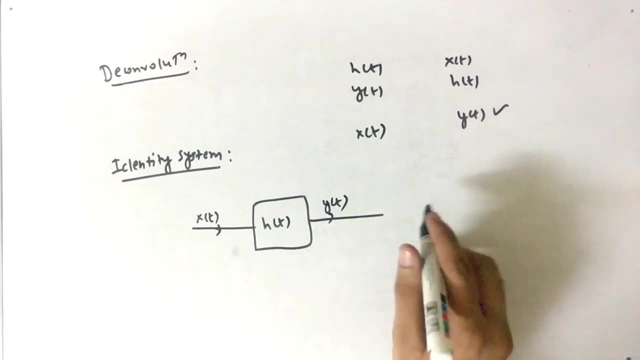 So this is a system where you give input x of t and the impulse response is h of t and the output you get is y of t. Now, if this is the input of another system, So another system is this. Now, this is the inverse system. As you can see, y of t is input and you will